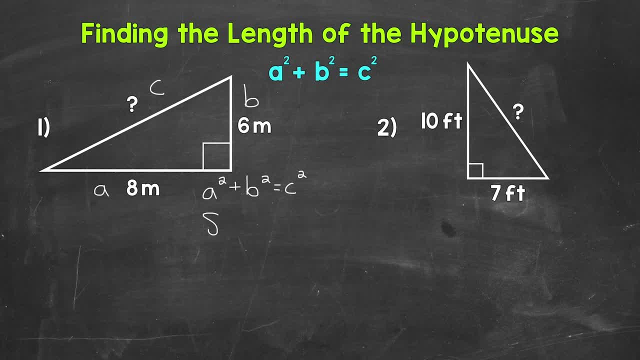 A is 8 meters, so let's plug in 8 for A. so 8 squared plus B is 6 meters, so plug in 6 for B, so 6 squared equals C squared. 8 squared gives us 64, plus 6 squared gives us 36.. 64 plus 36 is 100, so 100 equals C squared. 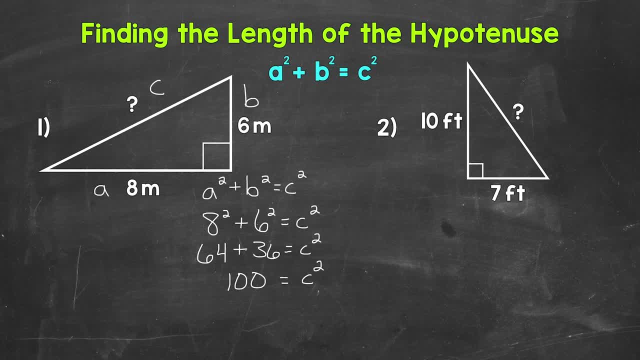 Our next step is to isolate C in order to figure out what C equals. So again, we are just working through this equation to figure out. Since C is being squared, let's take the square root in order to isolate C. Whatever we do to one side of the equation, we must do to the other, so we need the square root of 100 as well. 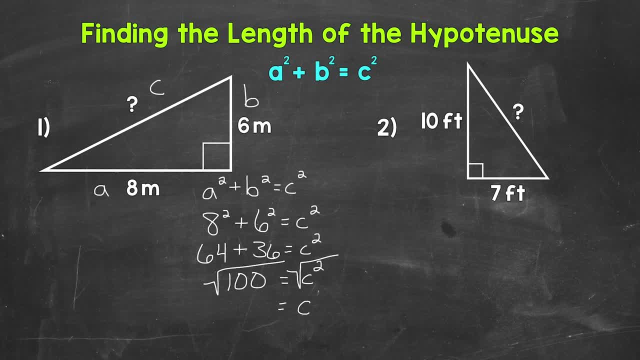 C is now isolated, so we have C equals. and then the square root of 100 is 10,, so C equals 10.. Let's rewrite that with C. We have C coming first, so C equals 10, and this is meters. 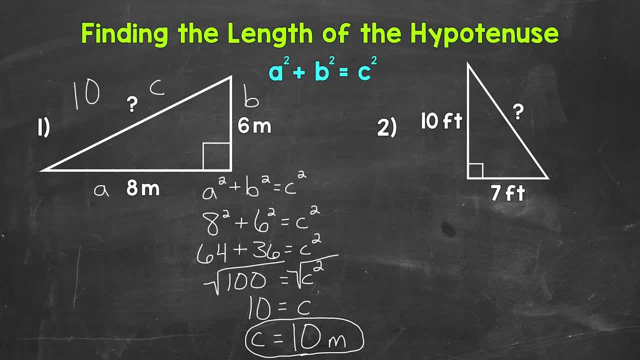 So the hypotenuse measures 10 meters and that's our missing side length. Let's move on to number 2, where we have a right triangle and again we need to find the length of the hypotenuse We are given the two legs. We have 10 feet and 7 feet. 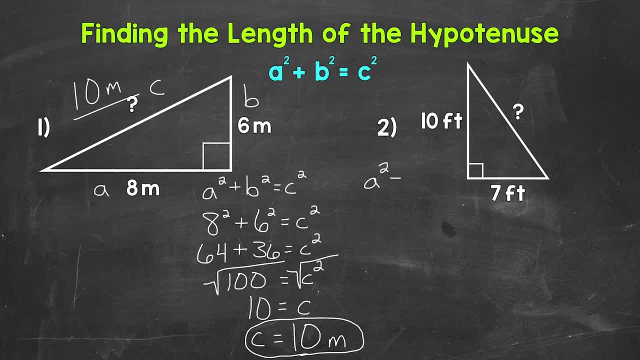 So let's use A squared plus B squared equals C squared in order to find the hypotenuse. Let's call this leg A, this leg B, and then the hypotenuse is C. Now we can plug in and work through this equation. 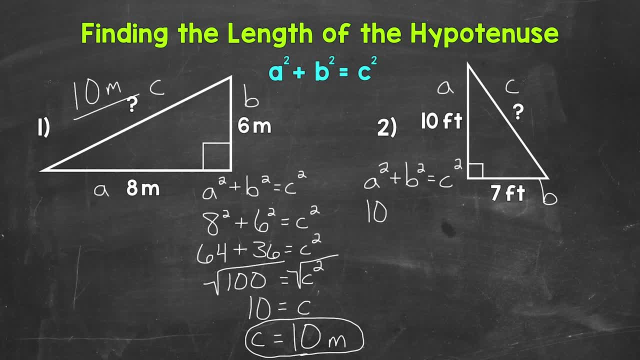 So for A we have 10 feet. Plug in 10 for A, so 10 squared, Plus 7 feet for B. So plug in 7 for B. 7 squared equals C squared. 10 squared, that's 100, plus 7 squared, that's 49, equals C squared. 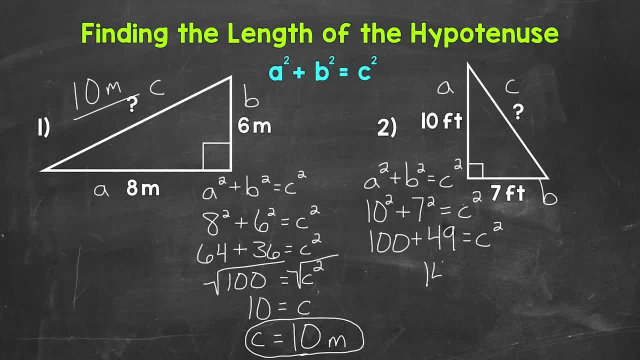 100 plus 49,. that gives us 149 equals C squared. Now we have 149 equals C squared, So our next step as we work through this equation is to isolate C. C is being squared, so let's take the square root in order to isolate C. 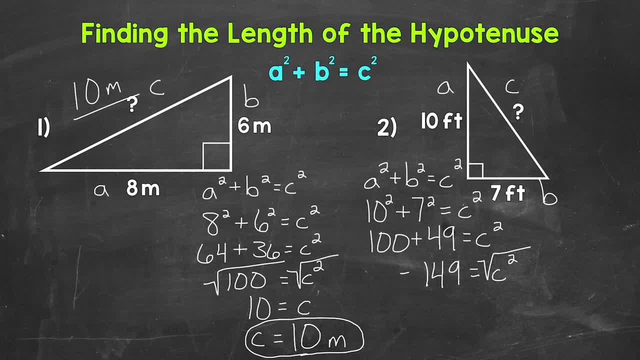 Whatever we do to one side of the equation, we must do to the other. So let's take the square root of 149 as well. We end up with an isolated C on the right side of the equation, And then as far as the square root, 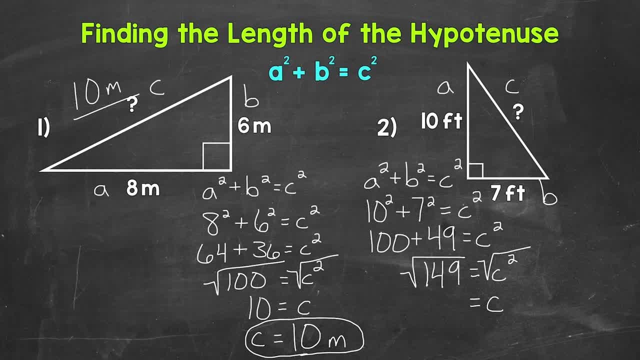 The square root of 149,. 149 is not a perfect square, So we do not end up with a whole number. answer C equals the square root of 149.. Now we can write the square root of 149 as an approximate rounded decimal. 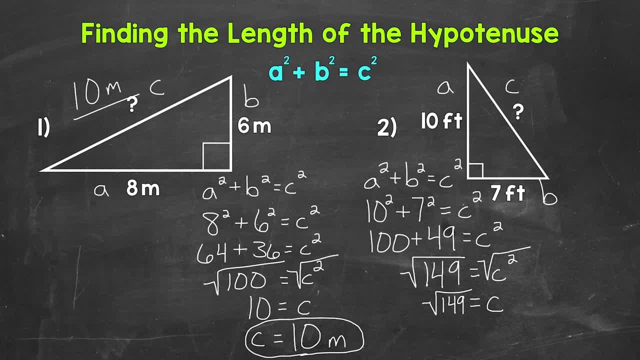 The square root of 149 is irrational. The decimal never stops and it doesn't repeat. So again, let's round it and we will round it. So the square root of 149 gives us 12.206.. And again, that just continues on. 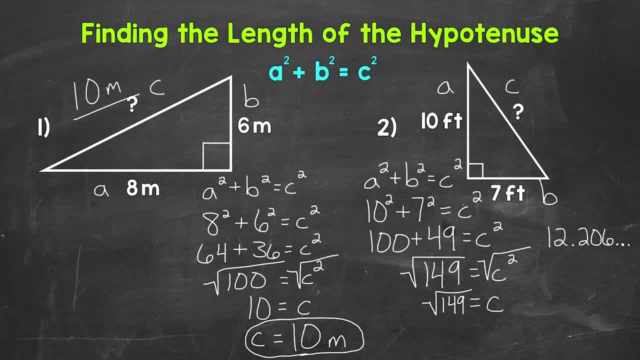 So I'm going to write it to the thousandths place and then round it to the hundredths. So let's round it to the hundredths place. We have a 6 to the right in the thousandths. so this rounds up. 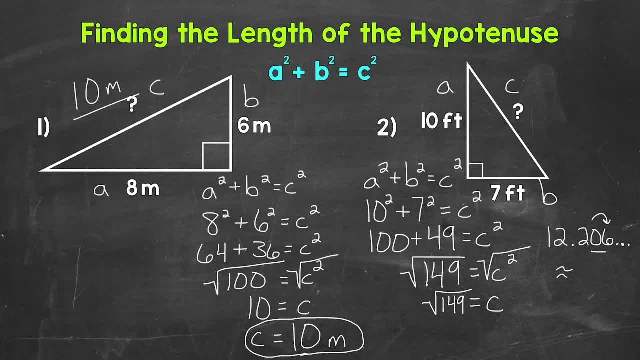 So the square root of 149.. 149 is approximately 12 and 21 hundredths, So C is approximately 12 and 21 hundredths and this is feet. So the hypotenuse is approximately 12 and 21 hundredths. 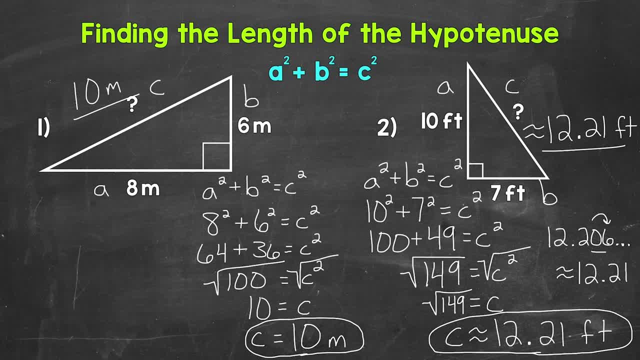 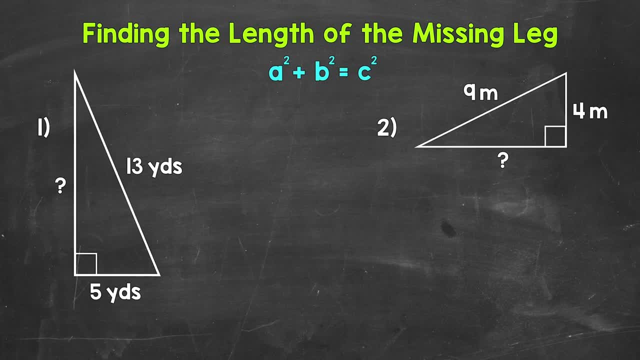 Again, this is feet, So there's how to find the length of the hypotenuse. Let's move on to finding the length of a leg. Here are a couple of right triangles and we need to find the length of a missing leg. 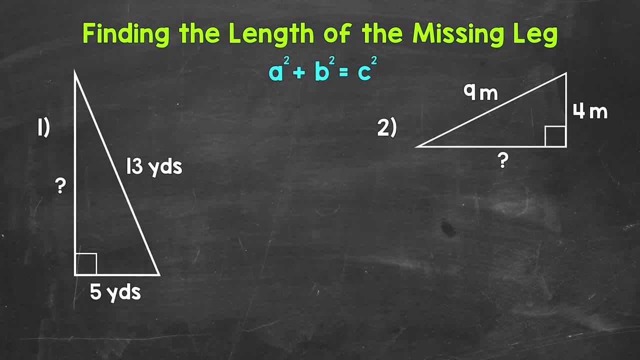 Let's jump into our examples, starting with number one, where we have a right triangle with one of the legs given and then the hypotenuse given. So one of the legs measures 5 yards and then the hypotenuse measures 13 yards. 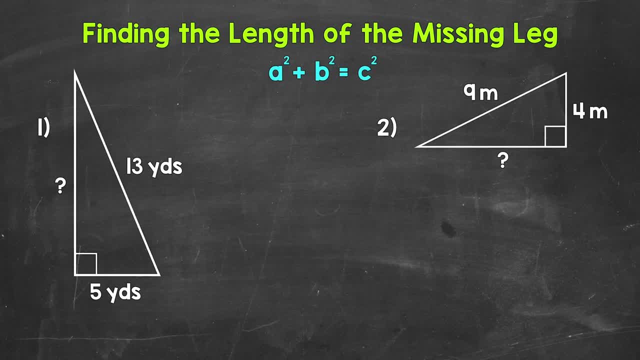 We need to find the length. We need to find the length of the missing leg. We're going to use a squared plus b squared equals c squared in order to find the length of that missing leg. Now, as far as that right triangle, let's call this leg a and this leg b. 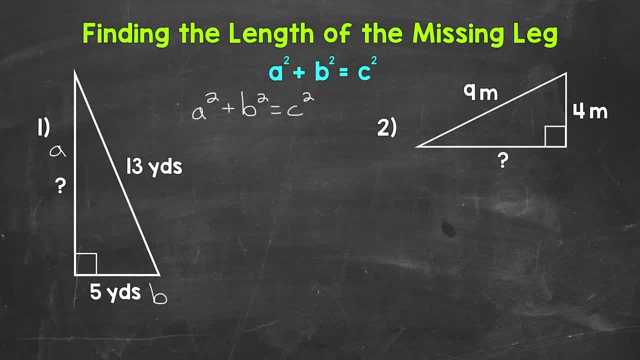 Remember, it doesn't matter which leg is a and which is b, and then the hypotenuse is always c. Now we can plug in what we need to plug in. We are given and work through this equation in order to find the length of the missing leg. 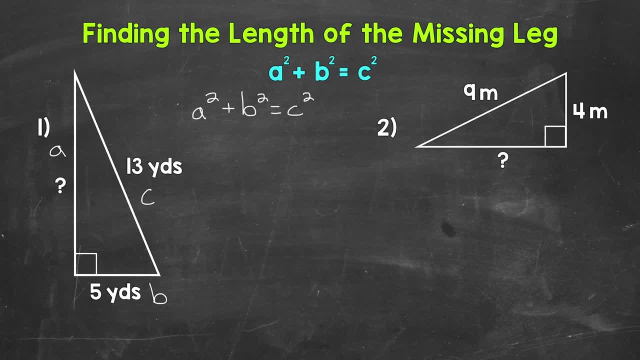 Now a is the missing leg, so let's keep this as a squared plus b squared. Well, b is 5 yards, so let's plug in 5,. so 5 squared equals: well, c is 13 yards, so let's plug in 13, and this is squared. 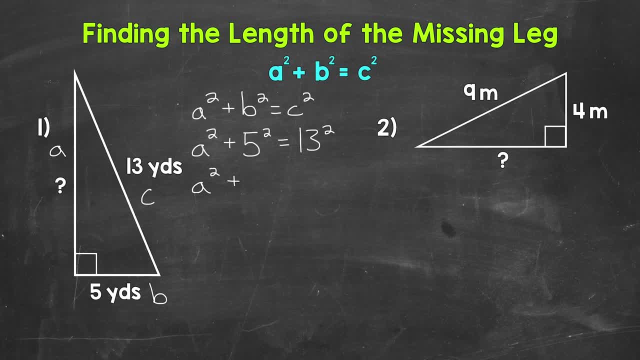 So that gives us a squared. Now, a squared plus 5 squared gives us 25, equals 13 squared gives us 169.. So let's continue on working through this equation and we are working to isolate a, We are working to figure out what a equals 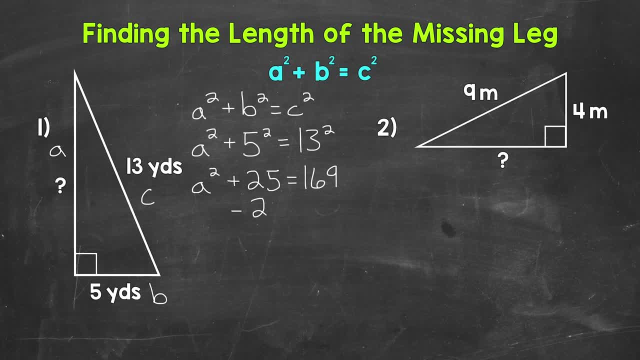 Let's subtract 25 from this side, and whatever we do to one side of the equation, we must do to the other. So subtract 25.. 25 from the right side of the equation as well. The 25s on the left side of the equation cancel each other out, so we have a squared equals. 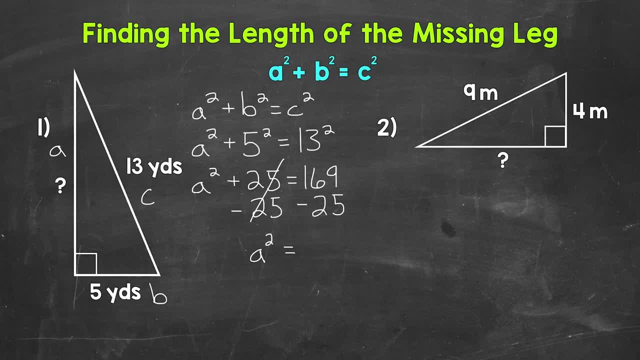 and then, on the right side of the equation, 169 minus 25 gives us 144.. So now we have a squared equals 144, and we need to continue to look to isolate a And figure out what a equals. Since a is being squared, we can take the square root in order to isolate a. 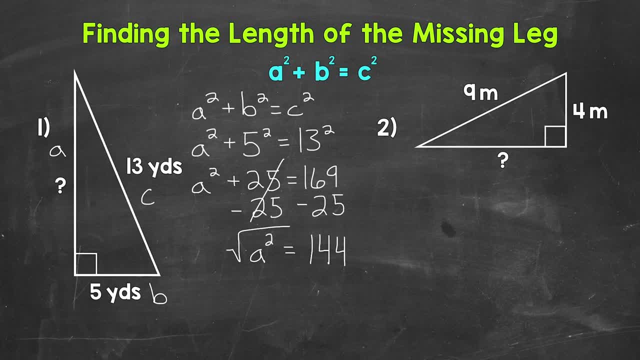 Whatever we do to one side of the equation, we must do to the other, So we need to take the square root of 144 as well. a is now isolated, so a equals: the square root of 144 is 12.. So a. 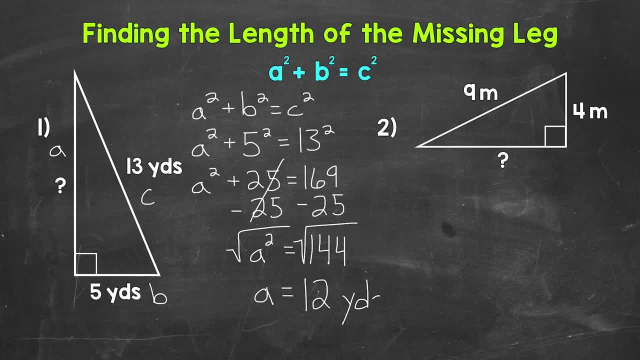 a equals 12, and this is yards. So the missing leg measures 12 yards. Let's move on to number two, where we have another right triangle and we need to find the length of the missing leg. We are given the hypotenuse, which is 9 meters, and then one of the legs, which is 4 meters. 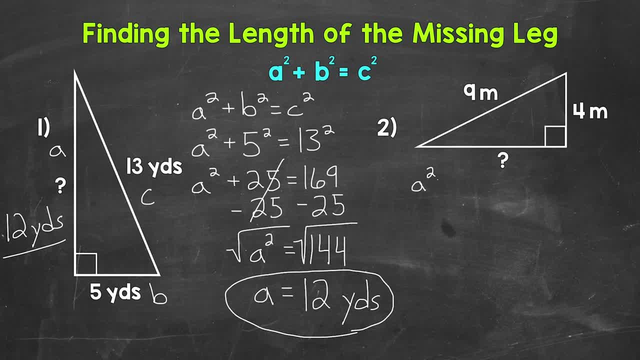 So let's use a squared. a squared plus b squared equals c squared. Let's call this leg a, this leg b, and then again the hypotenuse is always c. Now we need to plug in what we are given and work through the equation. 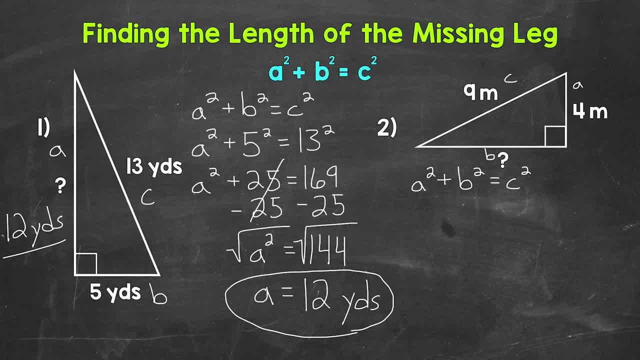 in order to find the length of the missing leg. So let's start with a squared. So we need a. a is 4 meters, so let's plug in 4.. So 4 squared plus b squared, Well, b is the missing leg. so let's keep this, as b squared equals c squared. 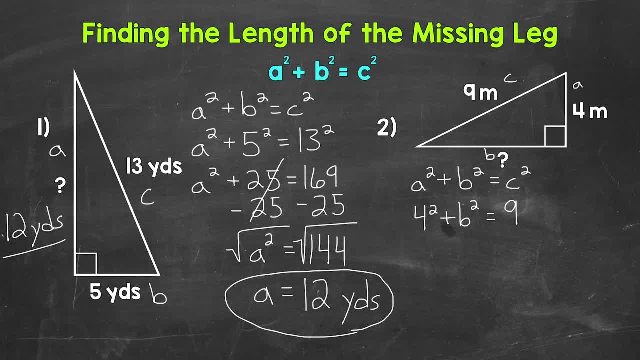 c is 9 meters, so plug in 9,, so 9 squared. Let's continue to work through this equation: 4 squared is 16 plus b squared equals well, 9 squared. So we need to plug in the missing leg and then again the hypotenuse is 81.. 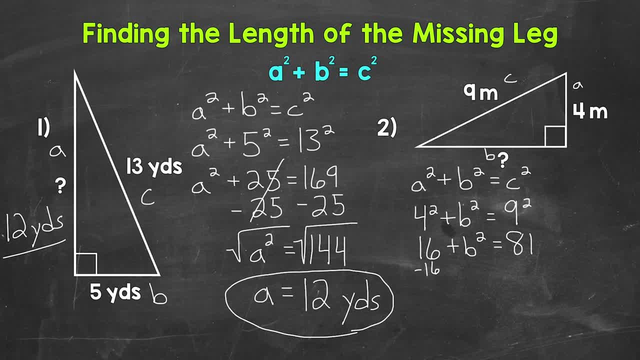 Now we can subtract 16 from the left side of the equation, And whatever we do to one side of the equation, we must do to the other. So let's subtract 16 from the right side as well. The 16s on the left side of the equation cancel each other out. 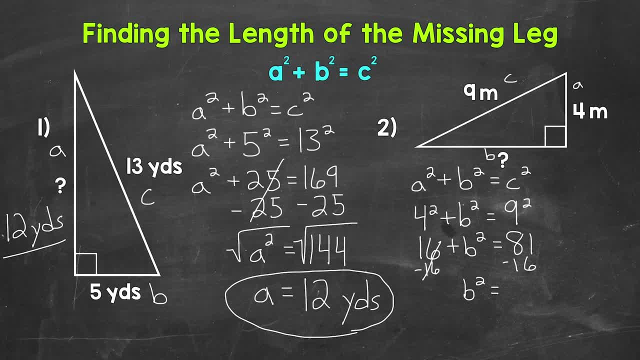 So we have b squared equals, and then 81 minus 16.. Gives us 65.. Since b is being squared, we can take the square root in order to isolate b. Whatever we do to one side, we must do to the other.